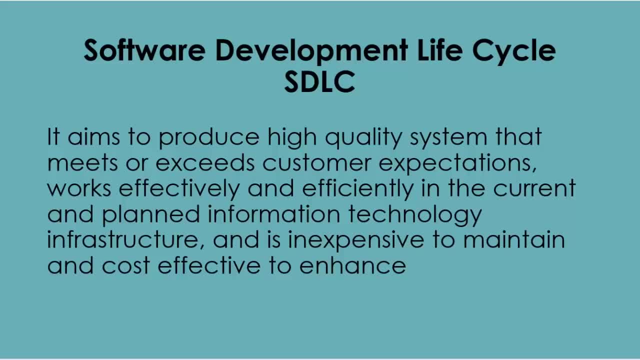 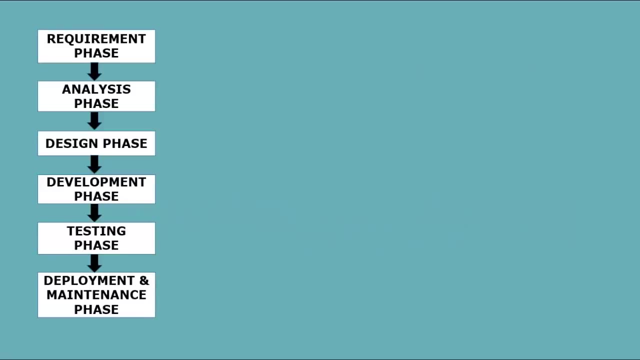 should be done on developed product based on requirement. Deployment should be done once the testing was completed. How to develop a product based on requirement. A typical Software Development Lifecycle consists of the following phases: 1.Requirement phase. 2.Analysis phase. 3.Design phase. 4.Development phase. 5.Testing phase. 6.Deployment. 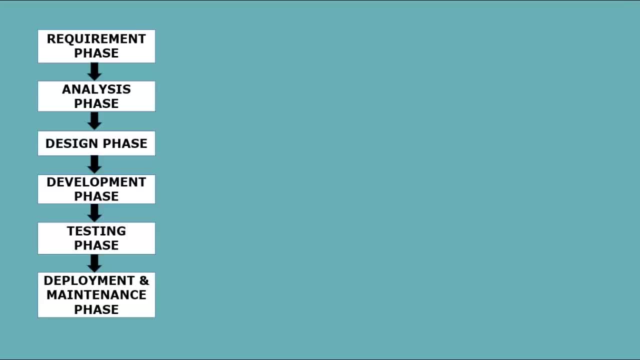 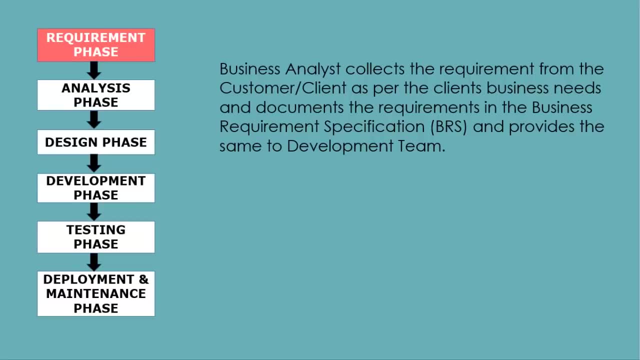 and Maintenance phase. Let's see each and every phase in detail: 1.Requirement phase. 2.Requirement phase. 3.Requirement Gathering and Analytics is the most important phase in the Software Development Lifecycle. 4.Business Enlist collects the requirements from our customer or client as per the client's. 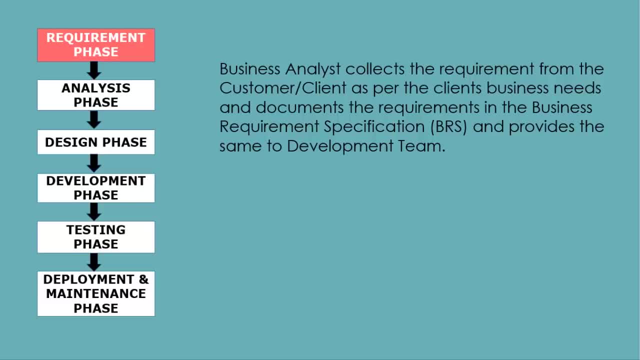 business needs and documents. the requirement in the business requirements specification, 5.Document Name varies. depends on team organization. Some examples: 1.Customer requirement specification. 2. Millennium document item. 3.C homework or CVS job certification. 4.Cusfacilitation of the product change. 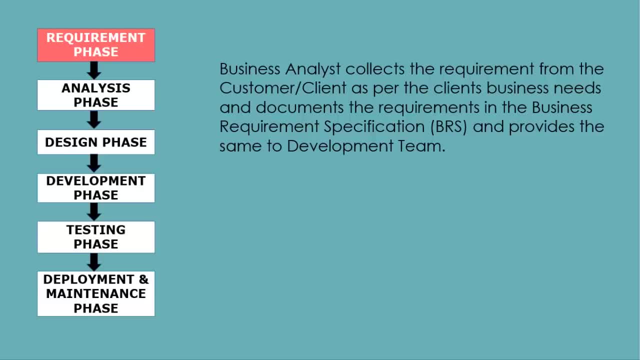 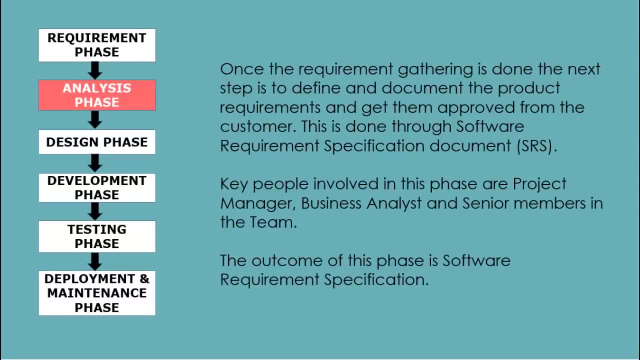 business specification, business requirement document, etc. and provides the same to the development team Analysis phase. Once the requirement gathering and analysis is done, the next step is to define and document the product requirements and get them approved from the customer. This is done through software requirement specification document. 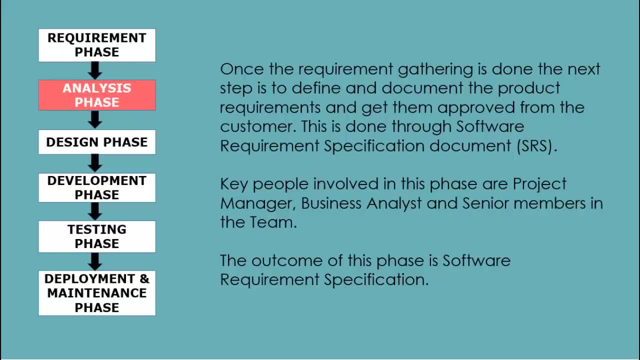 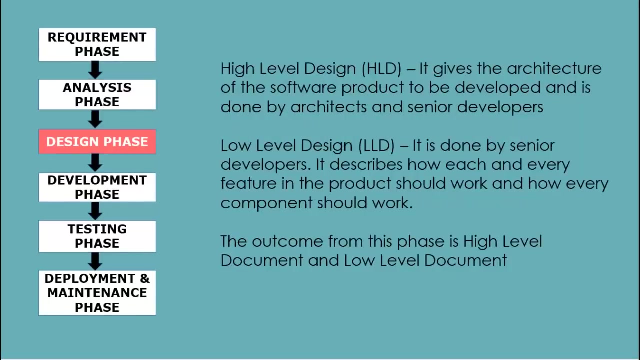 SRS consists of all the product requirements to be designed and developed during the project lifecycle. Key people involved in this phase are project manager, business analyst and senior members in the team. The outcome of this phase is software requirement specification Design phase. This phase has two steps: HLD- High level design. 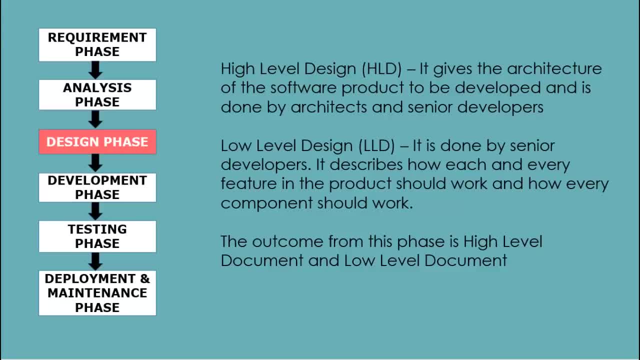 Design – It gives the architecture of the software product to be developed and is done by architects or senior developers. LLD – Low Level Design – It is done by senior developers. It describes how each and every feature in the product should work and how every component. 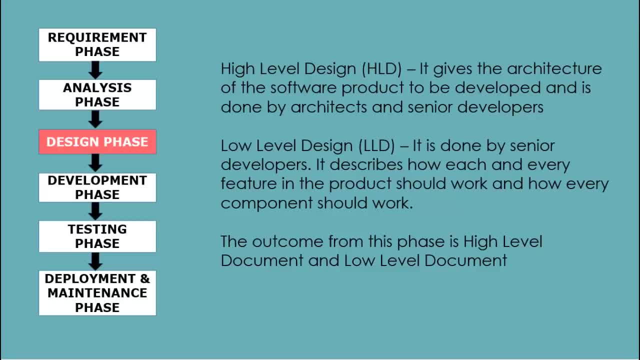 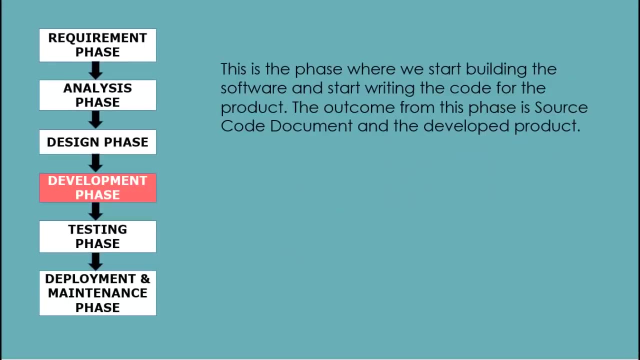 should work Here. only the design will be there and not the code. The outcome from this phase is high level document and low level document which works as an input to the next phase Development Phase – Developers of all levels- seniors, juniors, freshers- involved in this. 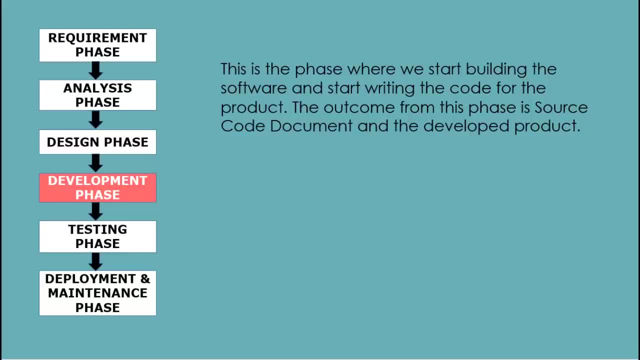 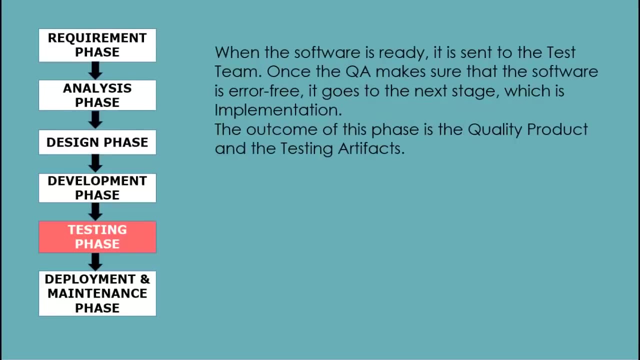 phase. This is the phase where we start building the software and start writing the code for the product. The outcome from this phase is source code document and the developed product Testing Phase – When the software is ready, it is sent to the testing department, where 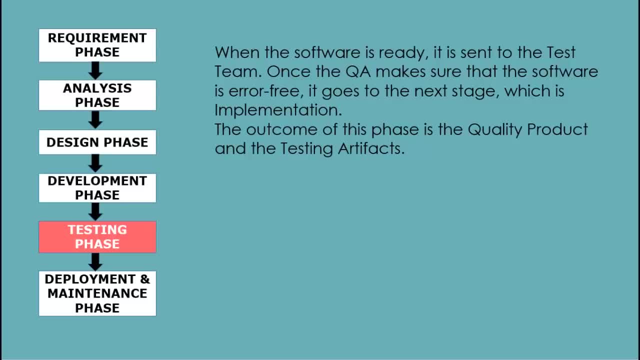 test team test it thoroughly. They either test the software manually or using automated testing tools- depends on process defined in STLC- and ensure that each and every component of the software works fine. Check out our video on STLC and its phases for clear understanding on how to test the. 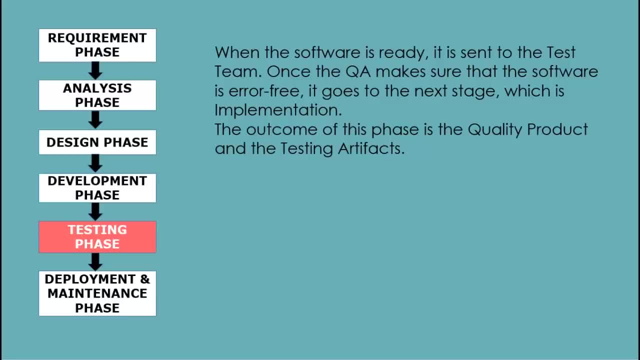 software. Once the QA makes sure that the software is error free, it goes to the next stage, which is implementation. The outcome of this phase is the quality product and the testing artefacts. Check out our video on test deliverables. We have discussed on list of the test artefacts we deliver in STLC. 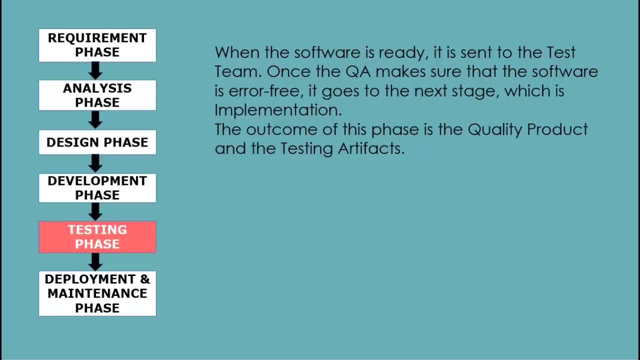 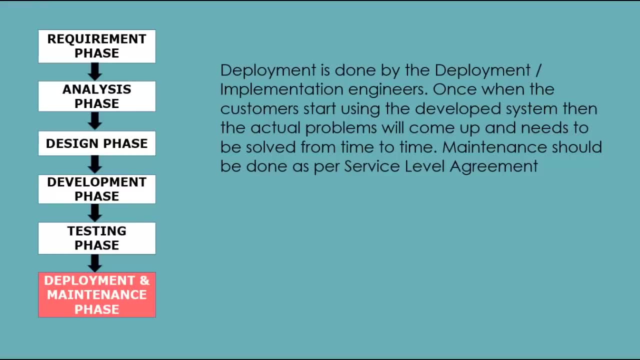 List out the test deliverables is one of the most popular interview questions. Deployment and Maintenance Phase – After successful testing, the product is delivered or deployed to the customer for their use. Deployment is done by the deployment or implementation engineers. Once, when the customer start using the developed system, then the actual problems will come. 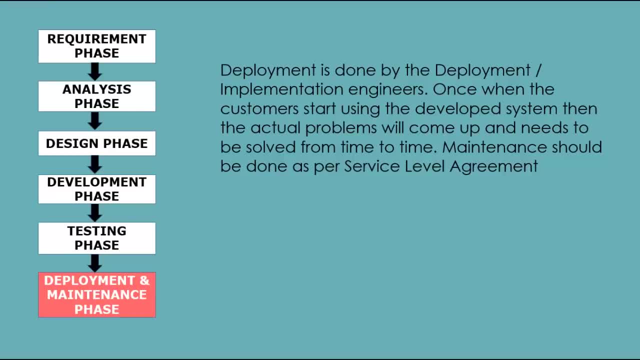 up and needs to be solved from time to time. The process where the care is taken is very simple. The care is taken for the developed product is known as maintenance. Hundred percent testing is not possible because the way testers test the product is different from the way customers use the product.